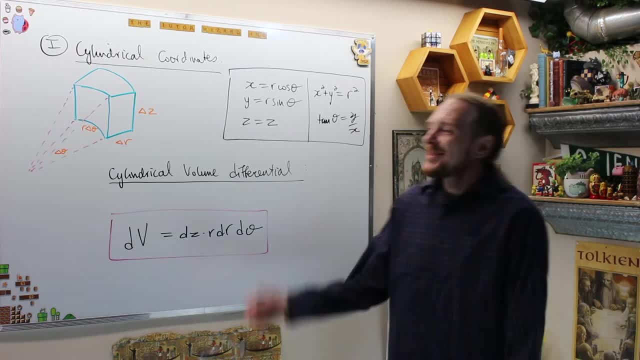 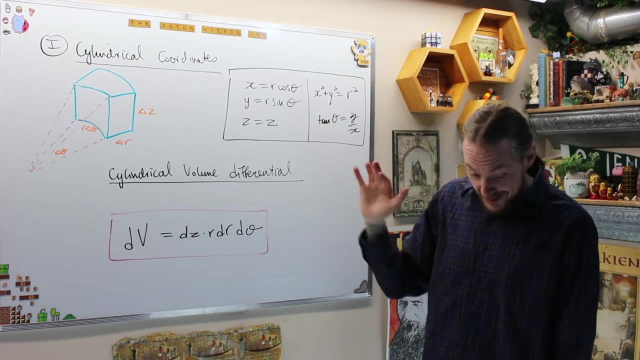 Let's do it. So. first we're going to do cylindrical coordinates. It's basically polar coordinates in three dimensions. We're just making it adding a tautology: z equals z. So we have x is r, cos theta, just like in polar, y is r. 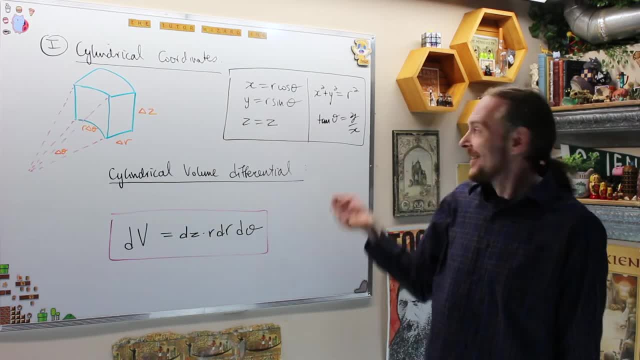 sin theta, just like in polar, and now z is z, z is just the height, and we also have the helping conversions that we want. x squared plus y squared is r squared, The reason we're doing this again. the bounds become much smoother when we translate everything from here, What we're now going to have. 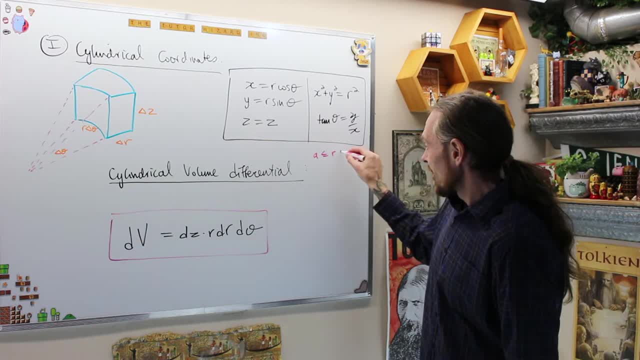 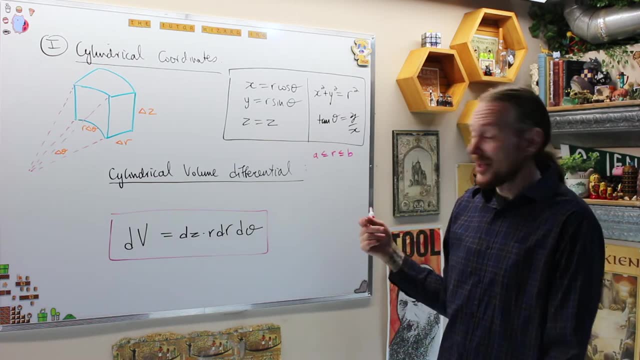 is, then we'll have- remember- a will be less than or equal to, r will less than b. most of the time You can change this r to be a general region of theta. Remember we did a polar coordinates, which we can do here also. but first take it easy and then you'll see that we're going to get out. 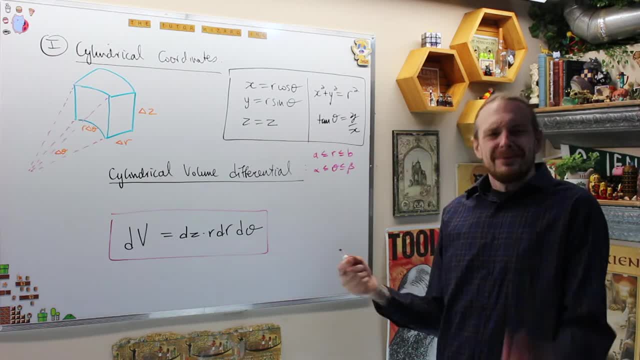 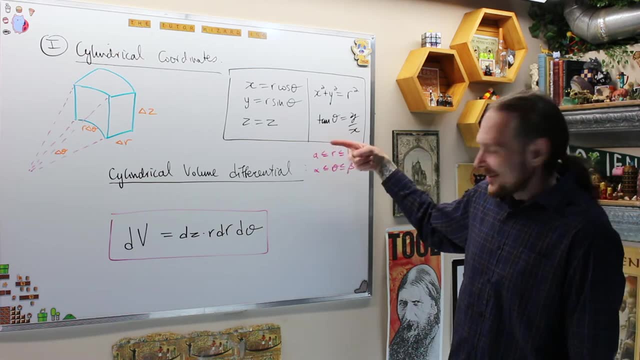 what is less than or equal to theta is less than or equal to beta. I know those all look like Greek to you anyways, which some of them are and some of them aren't Latin Greek, but these are numbers, Number, number, number, number. If we phrase it in another way: r squared is x squared plus y. 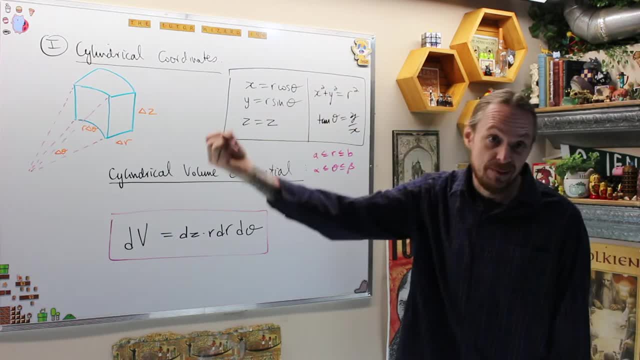 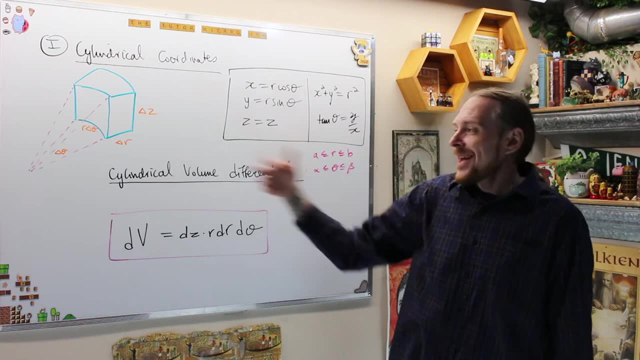 squared so you could have horrible functions in x, y or just have an r squared somewhere and this is why we start switching to cylindrical for certain shapes. When we do that quickly, we're going to do this in the last section of this chapter 2.8.. We're going to actually do change. 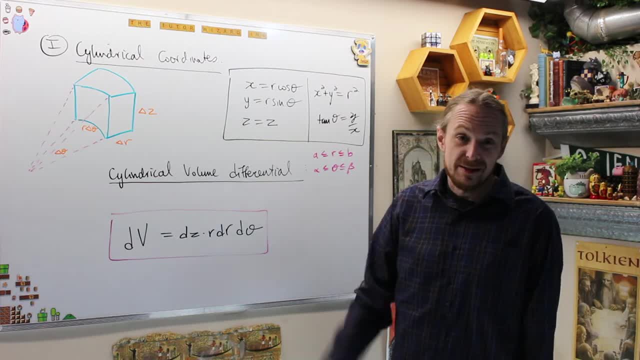 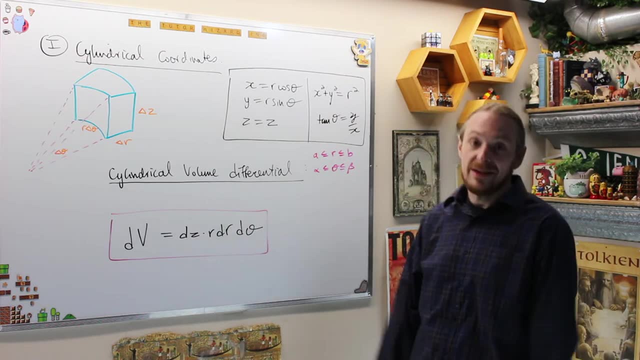 coordinate systems and look at all the differentials. if you do any change of coordinate system and it's translated: this r comes from the Jacobian that's going to turn out when we do this. so we'll discuss this in greater detail in the next section and in videos to come, but for now, 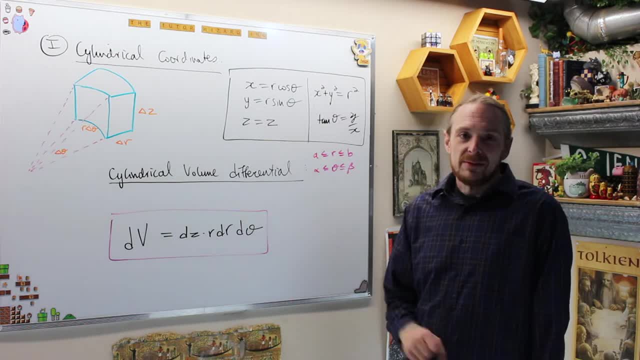 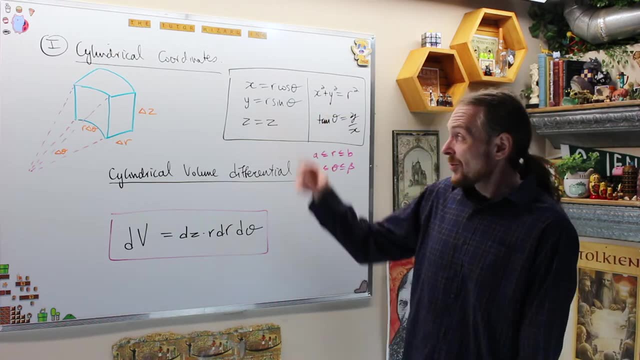 what we're going to do is just give you the volume differentials for cylindrical and spherical, and this is how we integrate in the change of coordinates. So if we want to change from Cartesian x, y, z, x equals x, y equals y and z equals z, to x equals r, cos theta, y equals r. 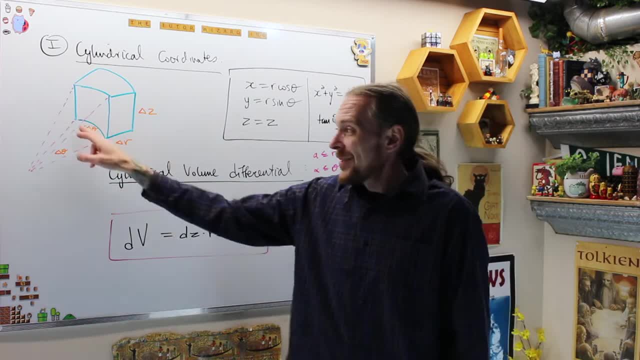 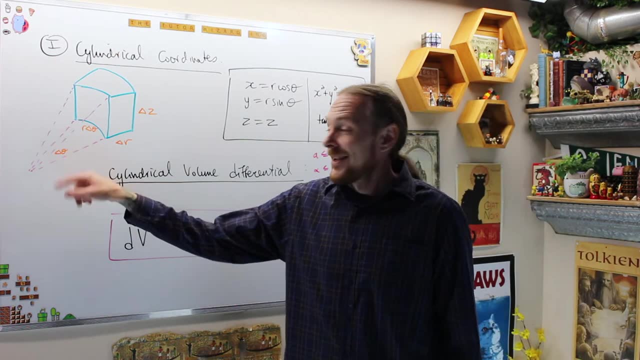 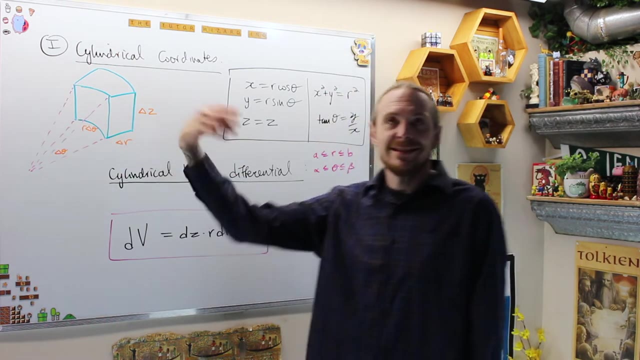 sine theta And z equals z. the differential we're going to get is because of the arc length subtended by a circle of length r and with angle theta. in this case it's delta theta. so the length s of this arc right here is not just delta theta, it's r delta theta. and that's where, in this derivation, 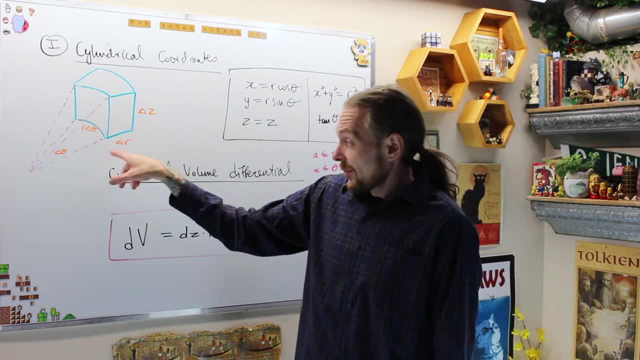 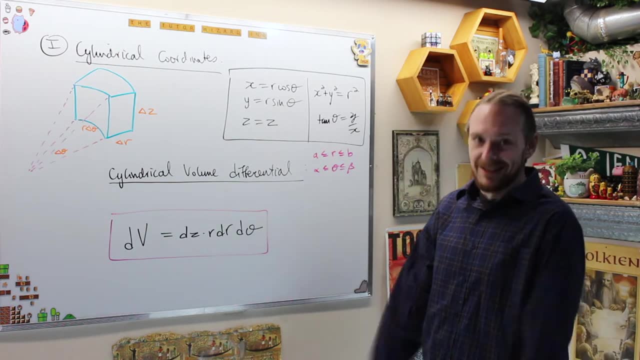 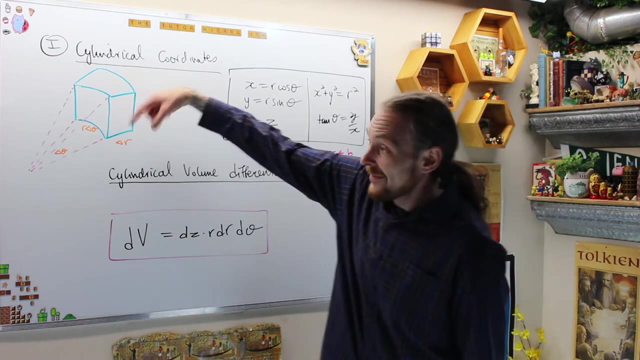 where that r is going to come from. it's from the Jacobian. and then, multiplying this volume of this differential box or this, what is this now? a polar rectangle, I guess, or a polar box. last time was a polar rectangle, this time it must be a polar cube or a polar box. the volume of that. 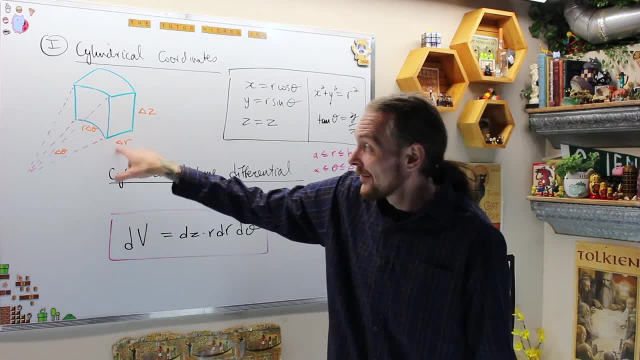 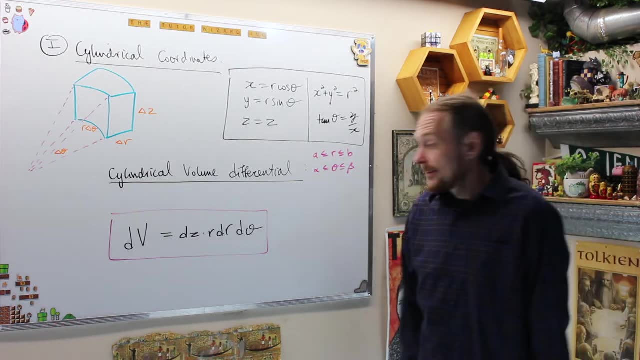 is going to be length times, width times, height again, and then we cleverly figure out what those are and this is where we get the cylindrical volume differential. let's do an example of this, all right example one: let's find the triple integral of z over this region, e, where e is the 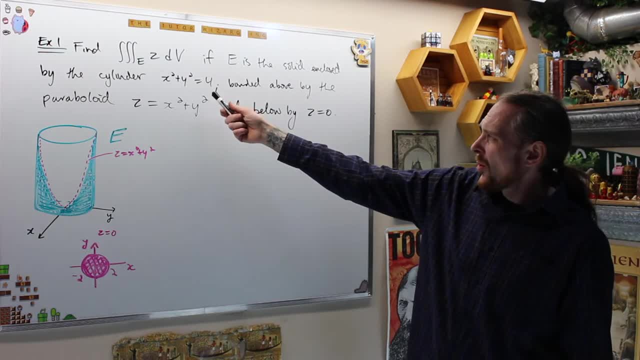 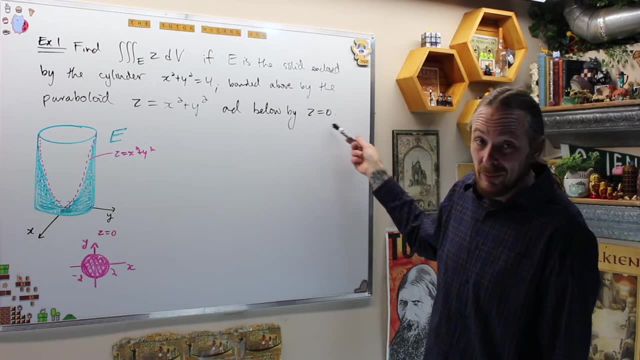 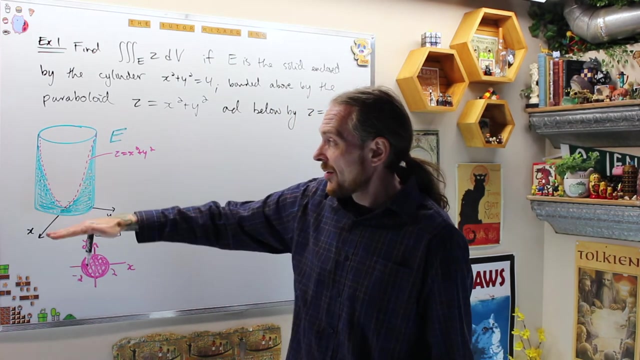 solid, enclosed by the cylinder- x squared plus y squared equals four- but then bounded above by the paraboloid- z equals x squared plus y squared- and below by the x? y plane, which is z equals zero. so we have z equals zero, the x y plane down here is where we stop, and then we we have the cylinder. 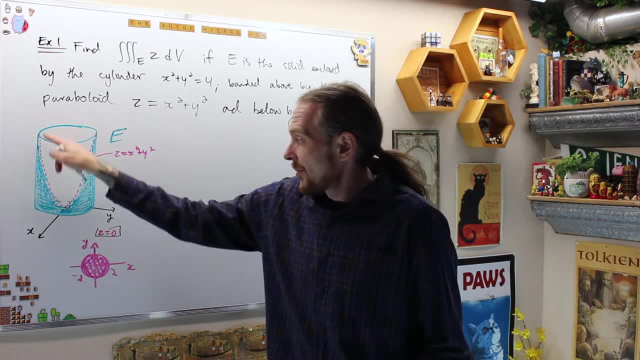 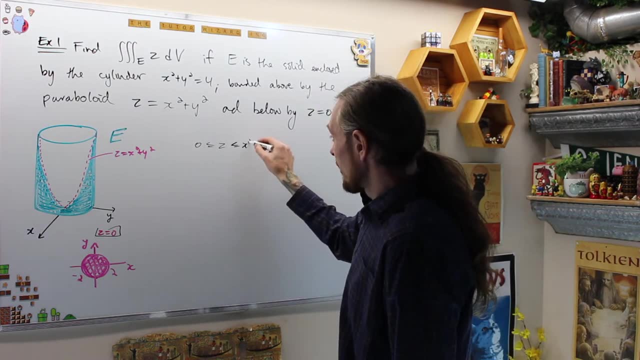 but it's bounded above by this paraboloid: z equals x squared plus y squared. so I already see that I'm going to have: z is less than or equal to zero is less than or equal to x squared plus y squared. but then I see I have that if I put that in spherical, that's going to say x squared plus. 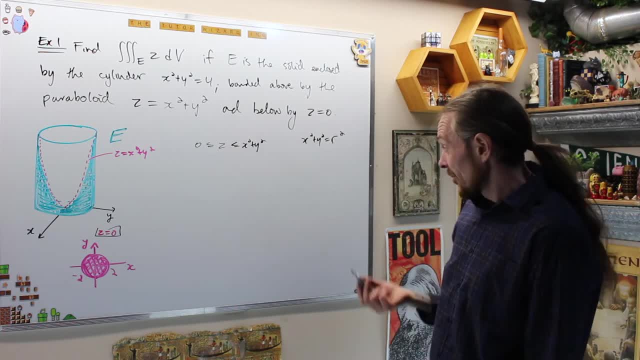 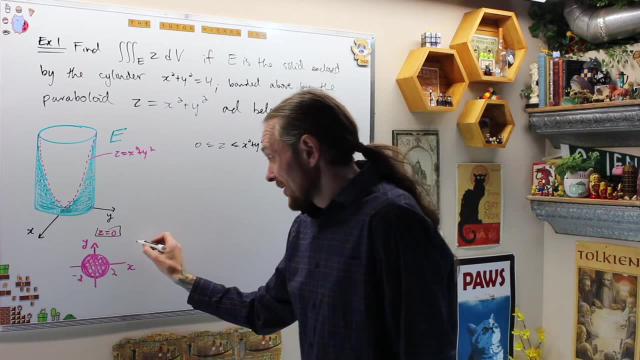 y squared is four For cylindrical, that's going to give me x squared, plus y squared is r squared, so that could immediately give me r squared for my bound. and then, when I look at this, it's nice to say that I'm going to have: zero is less than or equal to, r is less than or equal to two and zero is less. 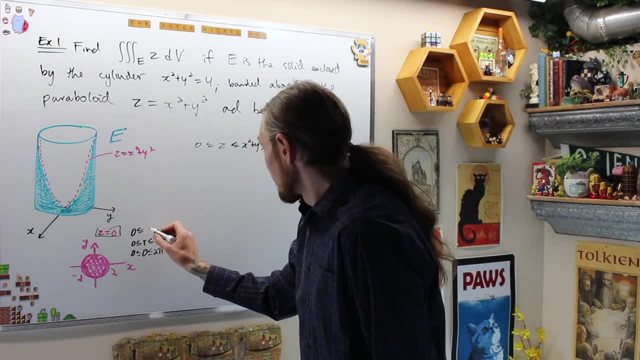 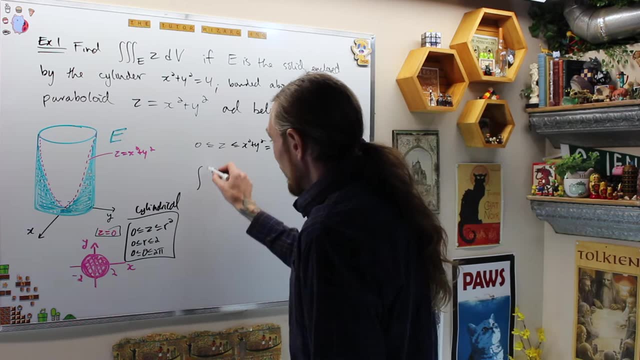 than or equal to. theta is less than or equal to two pi zero is less than or equal to. z is less than or equal to r squared. and these are my cylindrical. then what do I do with that? that says my triple integral over e of z, dv. z is z, so he stays. 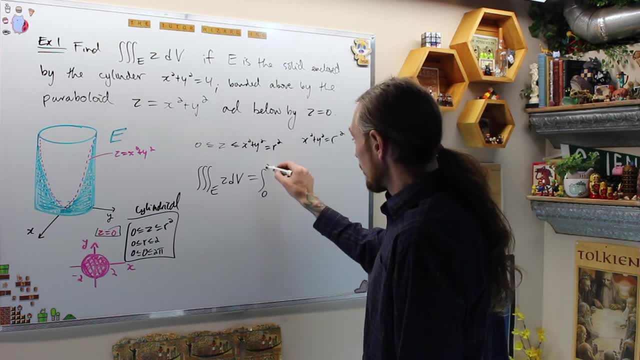 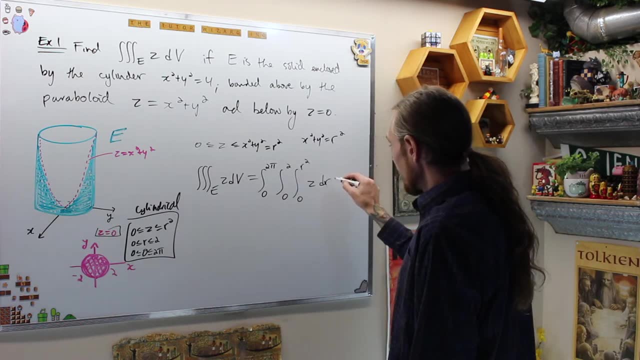 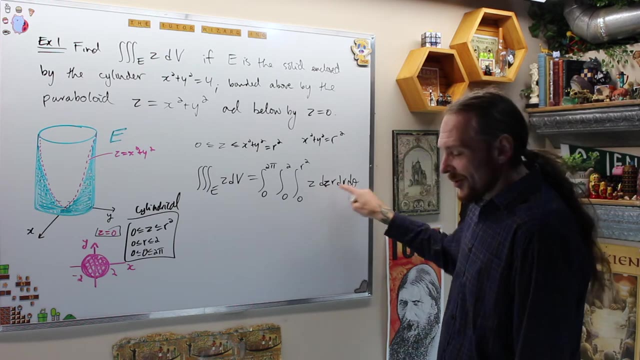 But everything else changes. this is the integral from zero to two pi, the integral from zero to two, the integral from zero to r, squared of z dr or dz r dr d theta. yes, it bothers you. these are all numbers so you can technically move them. it's going to go in here. this is equal to the integral. 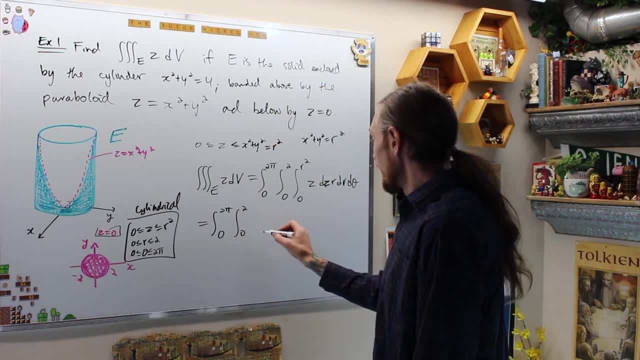 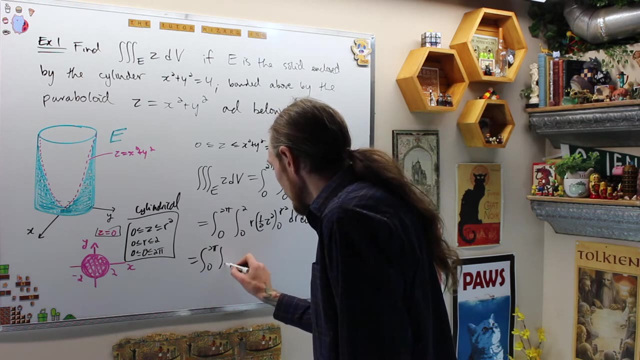 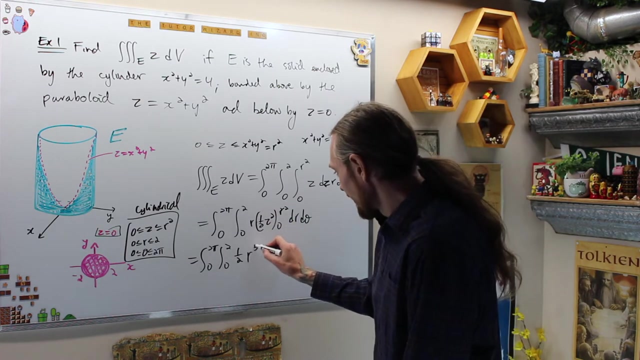 from zero to two pi, the integral from zero to two of r times one half z squared, evaluated from zero to r squared, dr d theta, this is equal to the integral from zero to two pi the integral from zero to two of one half r squared squared. and then I get another r, so r to the five, dr d theta. 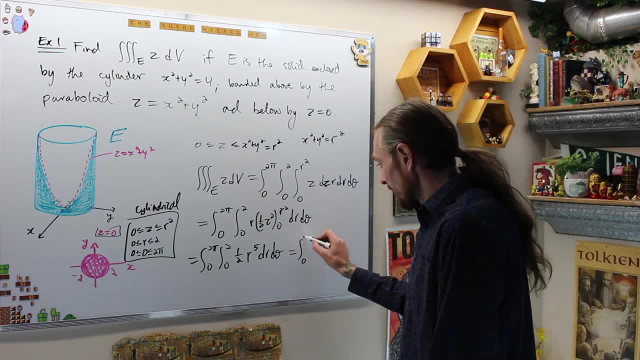 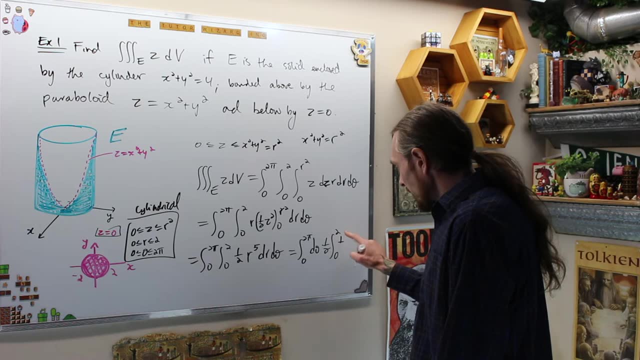 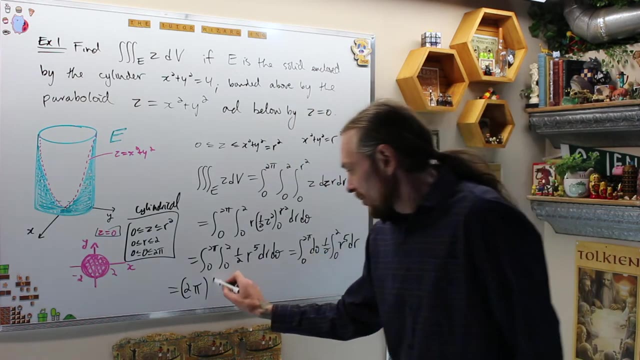 I can split that if I want. I'm going to do that. this is the integral from zero to two pi of d, theta times one half. the integral from zero to two of r to the five dr. this is equal to two pi, the first integral times one half, which cancels nicely. and then I'm 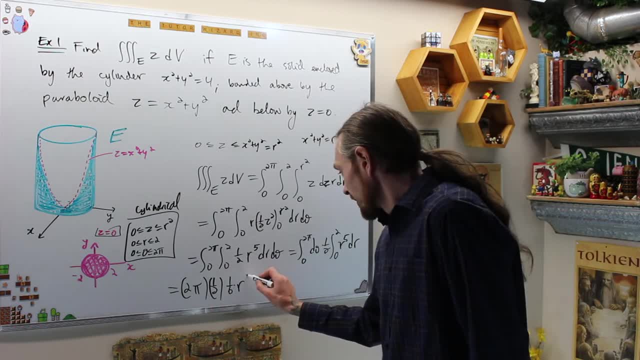 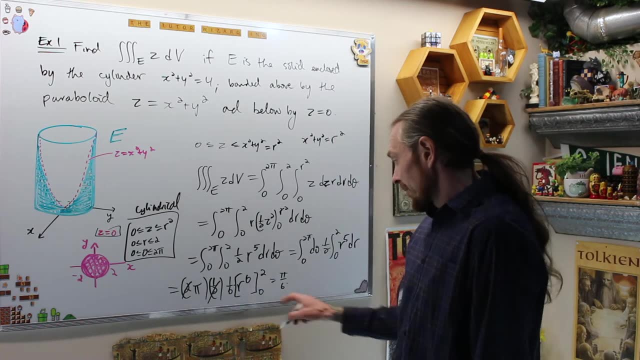 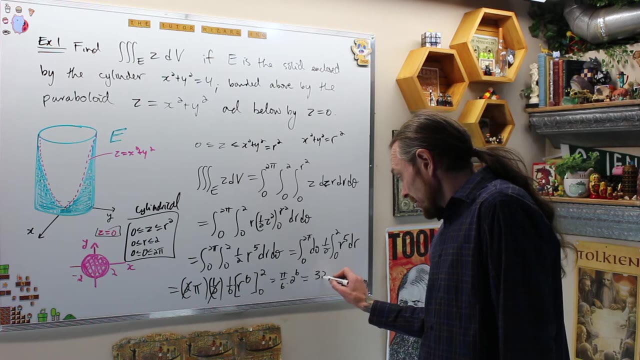 going to get one over six. r to the six, evaluated from zero to two. this cancels this cancels. this gives me pi over six times two to the six. there's a two in there, so I can cancel that. that's two to the five over three, which is thirty-two pi over three. 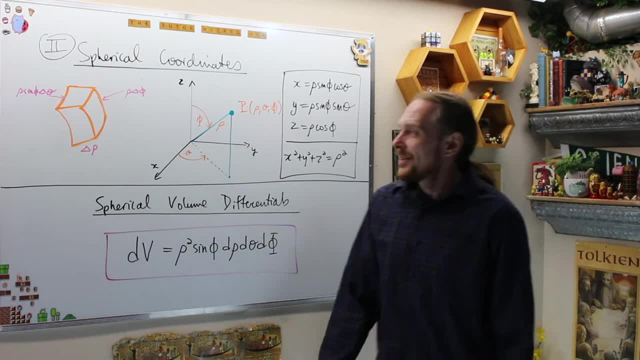 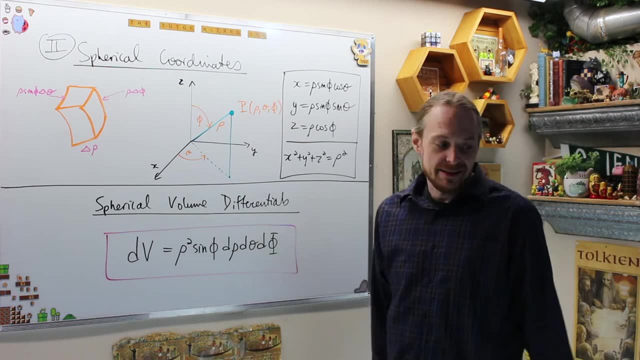 Let's do three. So if I want to change the spherical coordinates, then we'll do more for spherical coordinates. now again, we're going to do this in the next section of this chapter when we do change of coordinates for any kite type of coordinate system. you're like, why would you want to do that? because it's 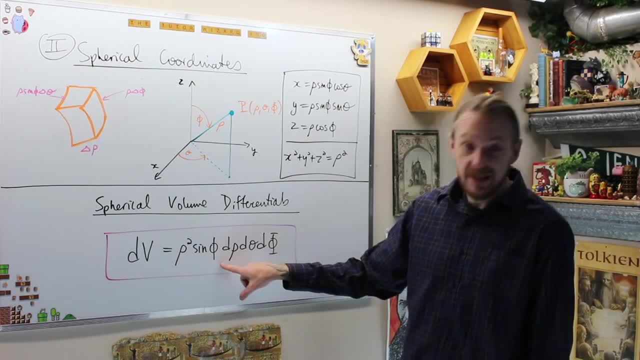 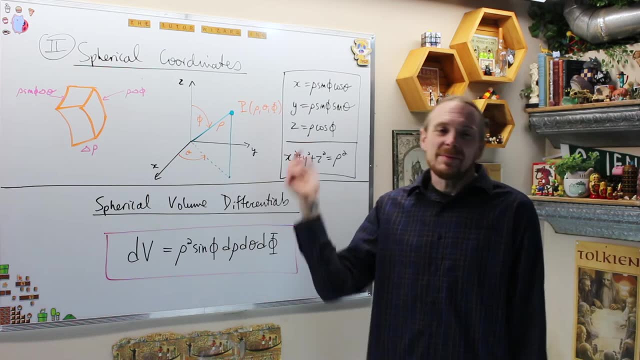 awesome. and then you get a Jacobian and you can carry around. these differentials will be phrased in terms of a Jacobian. right now, what we're doing is- this is fairly new to you- this one, cylindrical, is a little bit easier because you've seen polar already somewhere along the line. 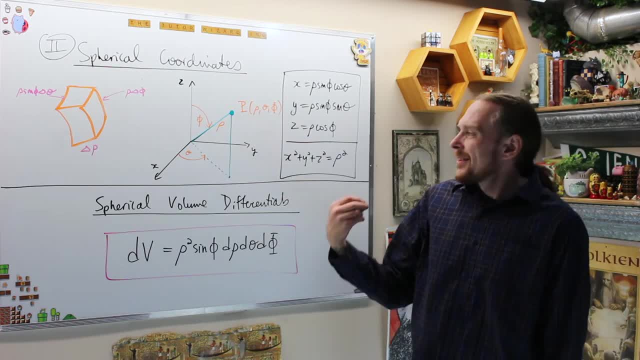 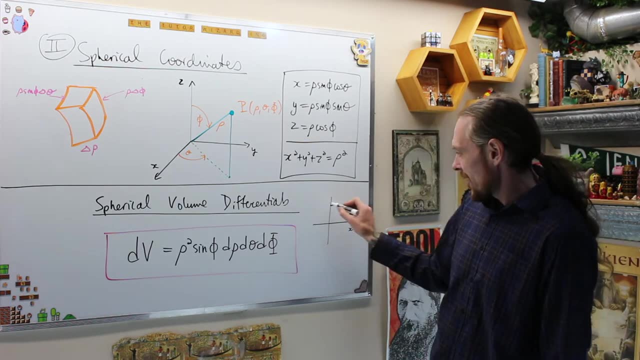 hopefully, but now this one. what we're rephrasing is every point in three space, just like in in the planar, in polar. what we're doing is every point. here you're used to phrasing as x and y, and then there's two pieces of information and we're going. 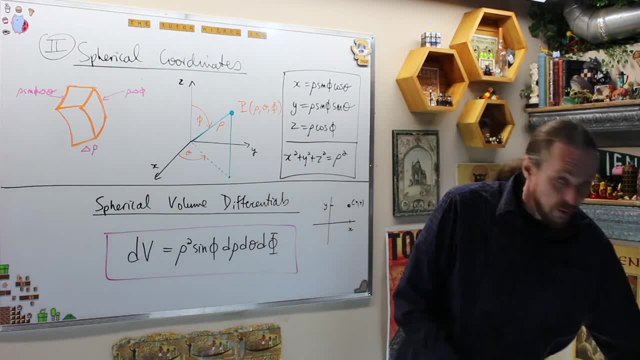 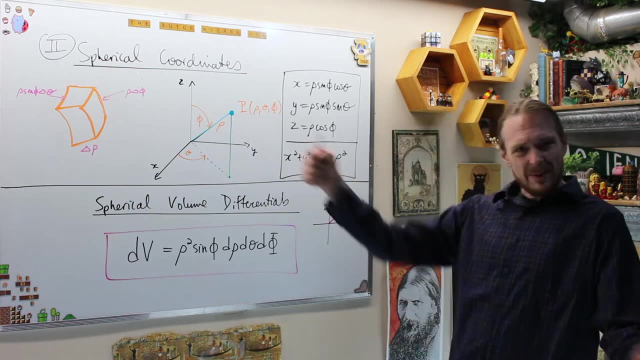 to call the coordinate xy in polar. what we're going to do now in polar says: well, you can do that, but I need two pieces of information, but not the same two pieces of information. if, as long as I know the radial distance from the origin and I know how far around I am in a unit, then those 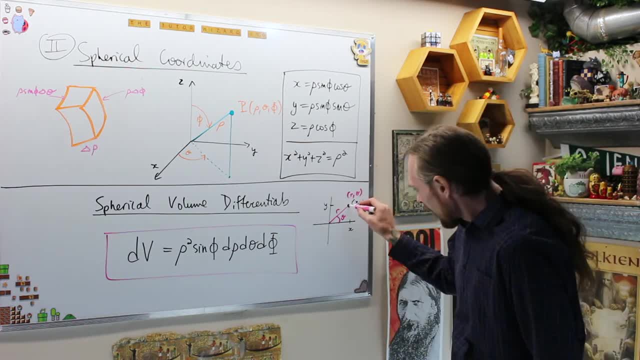 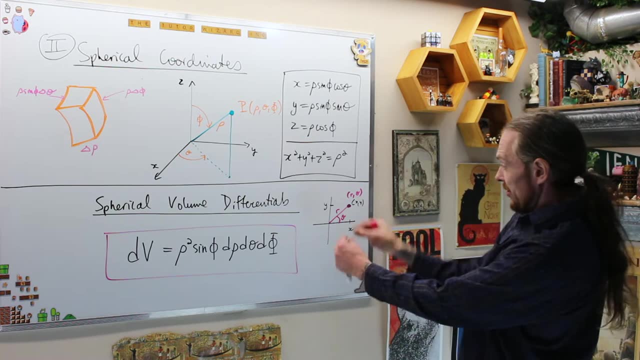 two people, pieces of information give me the same point in space. So I can describe every point in two space with Cartesian coordinates xy, or every point in space. how far out do I go and how far around do I go? I can get any point in space with polar coordinates. 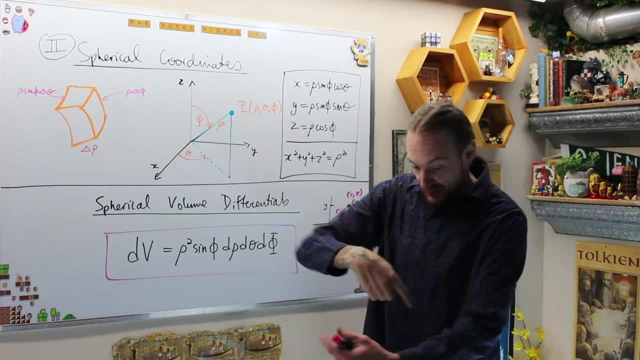 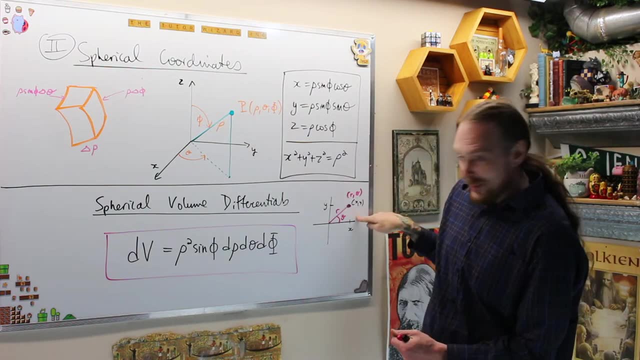 now we're doing the same thing with spherical, and now in three dimensions. what do I need? well, I need that radius. we're going to call it rho, possibly just to confuse you, because we like Greek, and not to be confused with the polar one, r then. so I need a radius out, then I need to be able to say how far. 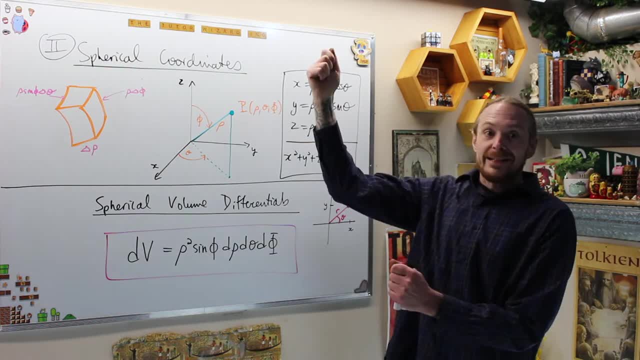 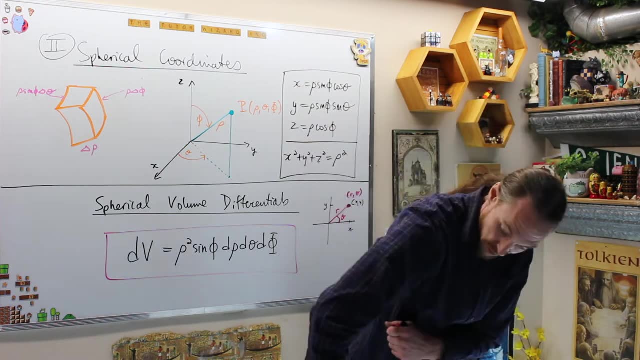 but now I have to talk about up and down, which I didn't have to do in the plane. so now all we're going to reference is of the vertical axis, and I can go from zero and phi is going to go from zero to pi is what our bounds for these three general regions are going to be. so in general, we're going. 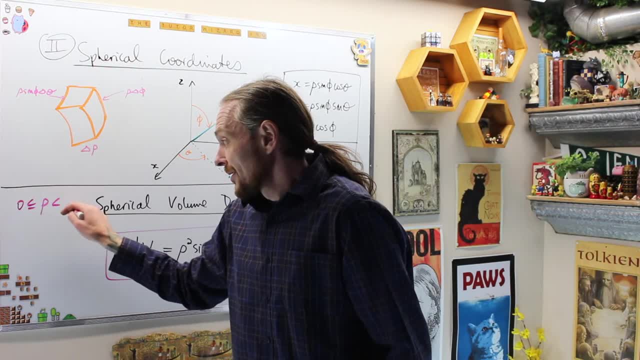 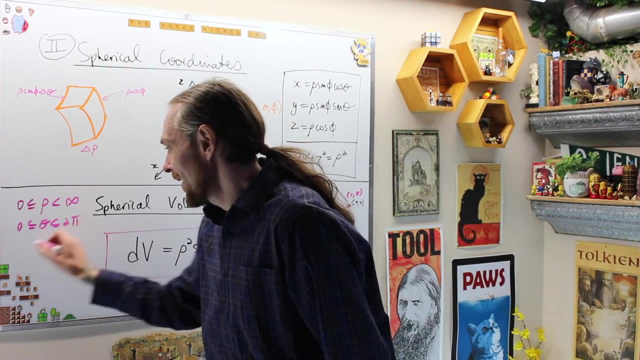 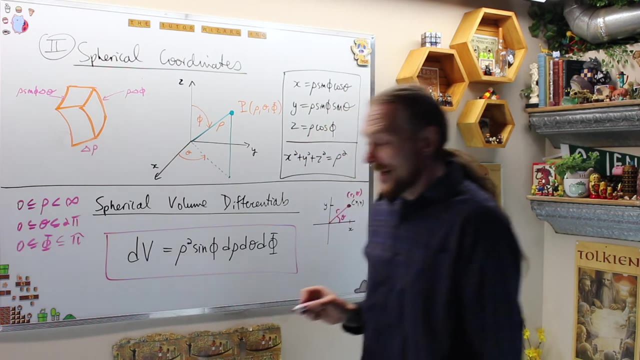 to have that zero is less than or equal to rho, is less than an infinity, some radius, and then we're going to have: zero is less than or equal to, theta is less than or equal to two pi, and zero is less than or equal to b, not phi. phi is less than or equal to pi radians. these are our general bounds. 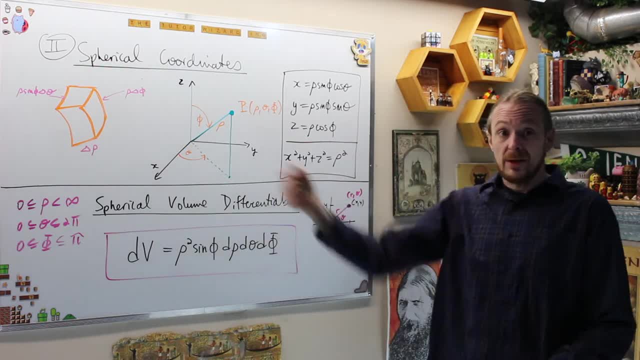 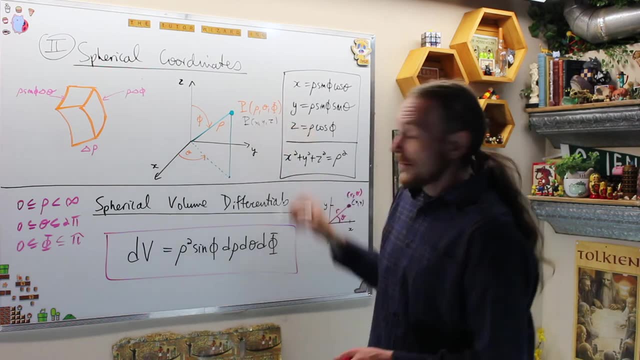 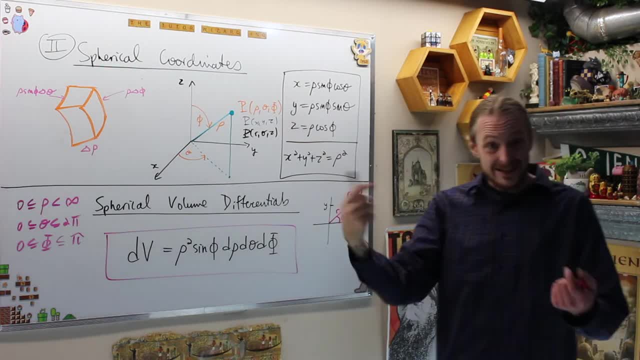 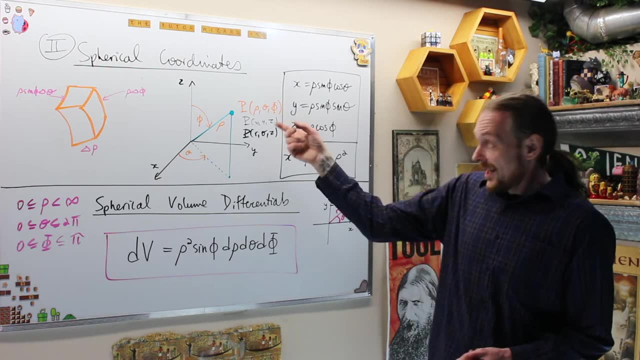 theta z, which was our cylindrical. now we have three ways of phrasing the same objects, but some of them are much more convenient when we want to triple, integrate and find volumes and all those kind of things. centroids- yeah, these ones are much more pleasurable to work with and 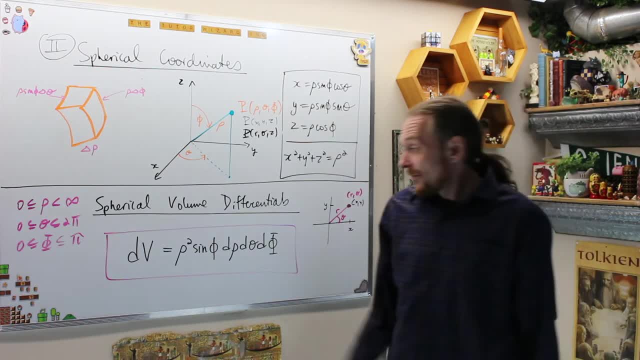 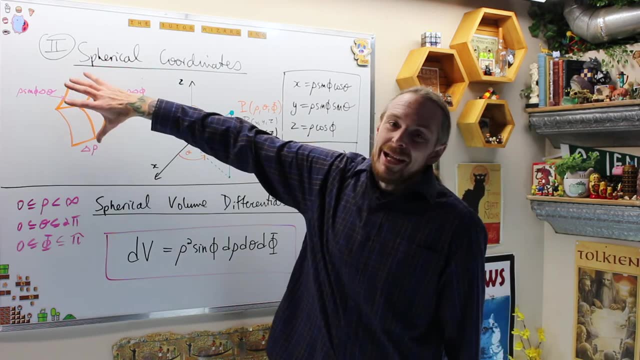 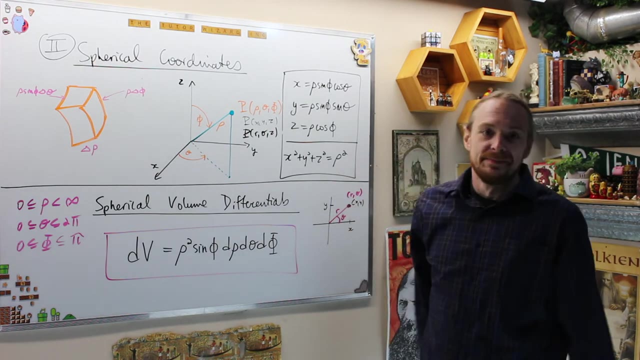 the bounds are nicer in certain scenarios. what is the differential volume for spherical coordinates in this derivation? again, we're going to do this in the next section, but the picture sort of gives us, if we have now a spherical box and we have two sides that are curvy, essentially what we're going to do is this one is the rectilinear one, that he's. 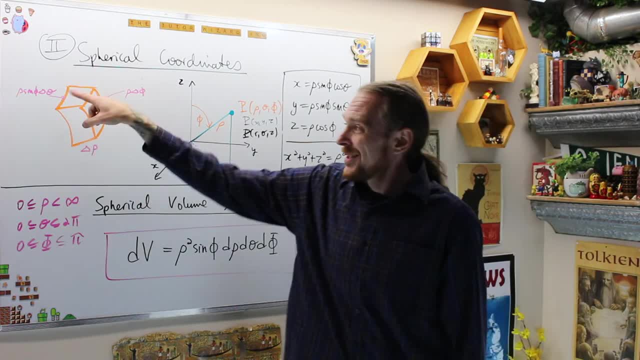 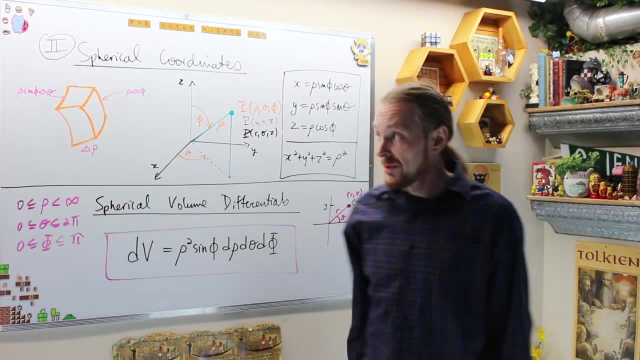 just a differential of the radius row. but now we have two little differentials. if we use some trigonometry and derive these or use Jacobians, we're going to find out that this guy is going to be equal to rho sine phi. small change in theta, remember. theta is going around and around this way. 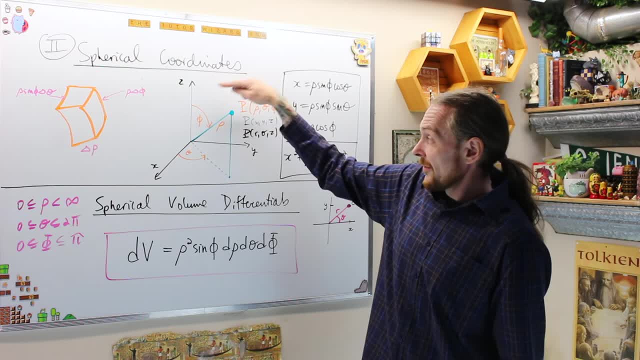 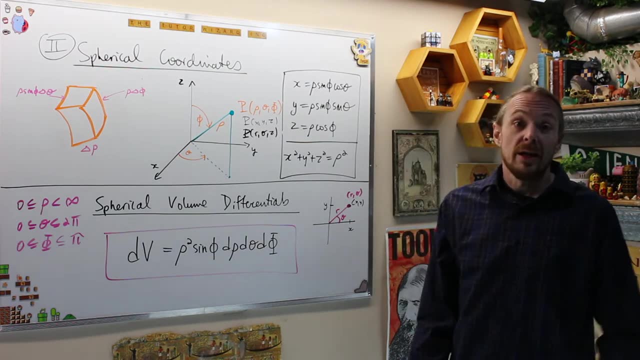 so it's a small change in theta. and then this one, finally, is the vertical. phi goes from here to here, so he's the vertical one. so this arc length is intended by that angle, which is going to be the radius row times, the small change in the angle. 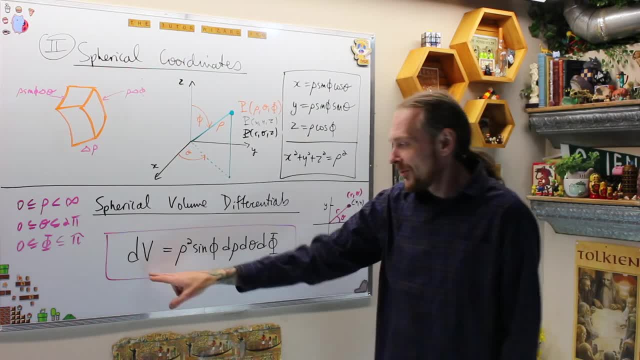 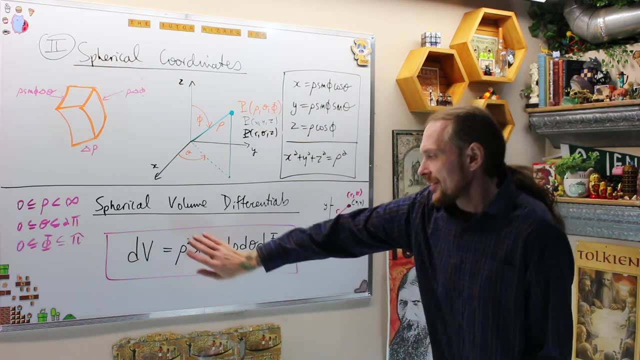 which is Delta B this time. putting that all together, we got the differential volume, we get row times, row, it's row squared, and then we have a sine B and we get that this differential is not just d? rho, d theta, d phi. we don't sound as cool and we don't sound like pirates anymore. it. 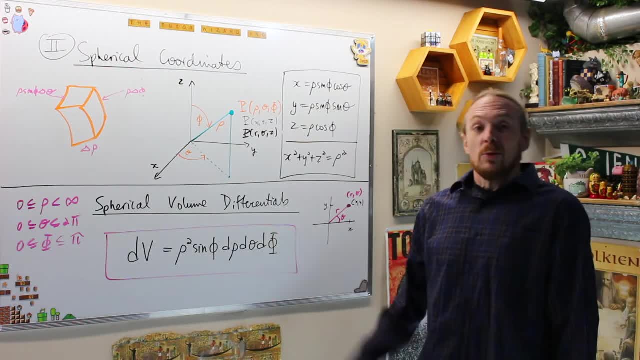 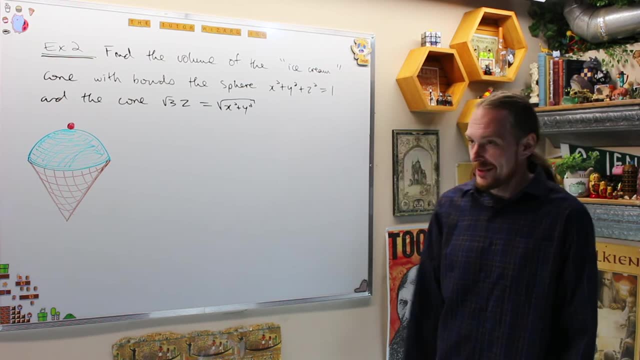 doesn't have quite the jingle. what is the differential? it's DV is rho squared sine phi d, no jingle. let's do an example. I really should have got the ice cream. now I want ice cream, so we gotta hurry up and finish this. this is literally the last scene you're gonna see me do the pitch. 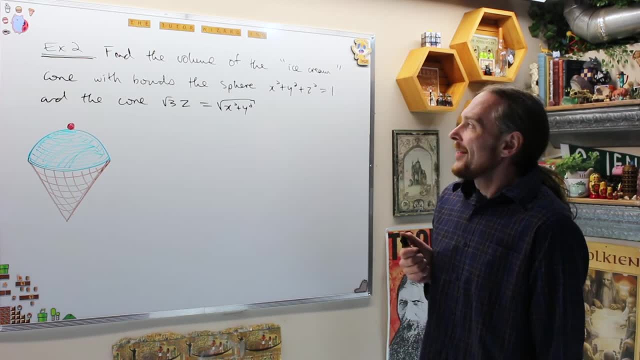 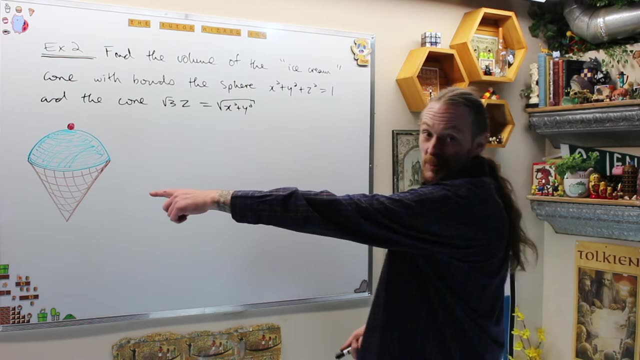 at the end. and then I'm gonna go eat ice cream. it's my daughter's birthday tomorrow. ice cream. find the volume of the ice cream cone bounded by the sphere. it's a perfect ice cream cone. you should see me make ice cream cones. perfect Spears, perfect wedge cones, and then we got a waffle cone. 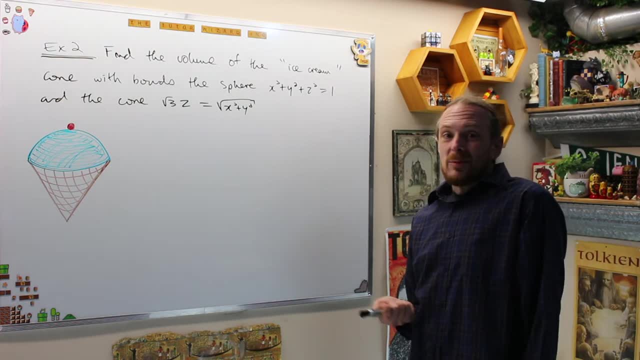 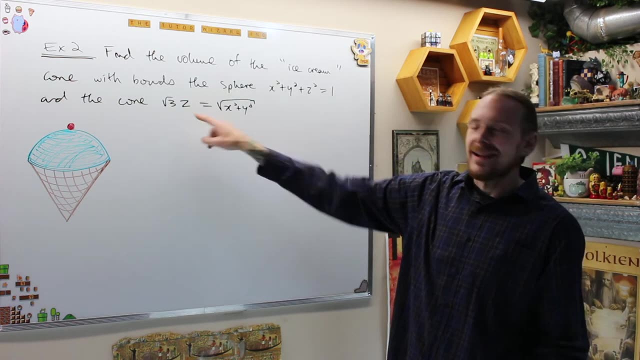 which is the cone root. 3z equals the square root of x squared plus y squared. I put the root 3 there so I could get a nice trigonometric value for myself. first of all, what is this going to look like in spherical coordinates? I'm gonna guess that, because I just did spherical. 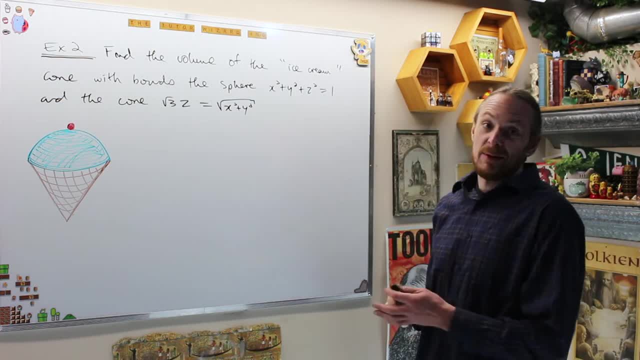 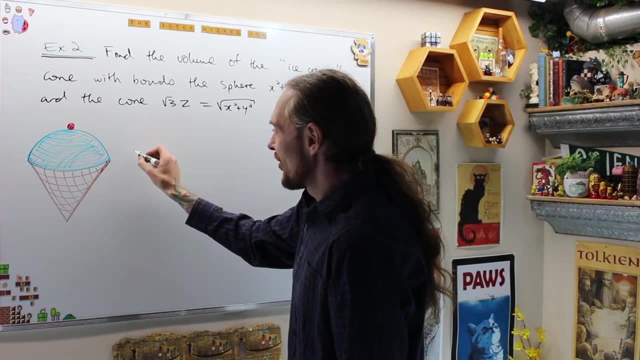 coordinates and I just said I'll, let's do an example. what am I going to use? probably spherical coordinates. what does that look like? in this right now I have, what does this guy look like? this one's not so bad, because we just get a conversion. we know that x squared plus y squared plus z squared. 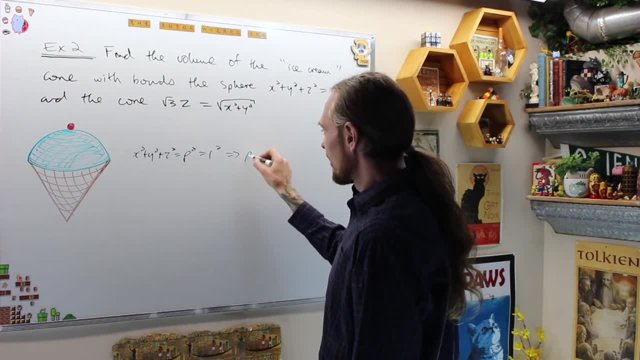 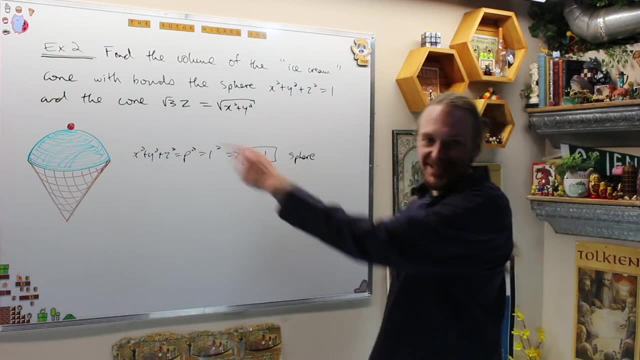 is rho squared and we're saying that's one squared. so that just says rho equals one. so that's what a sphere looks like in spherical. really easy. why do you think we're using coordinates? because it makes this equation as much as possible similar to integrate and do triple integrals and everything else. what's the cone? the cone is going. 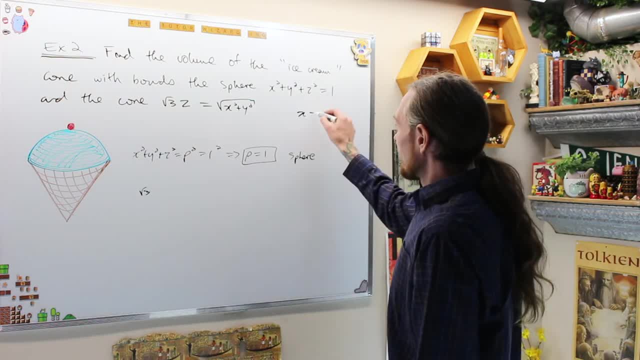 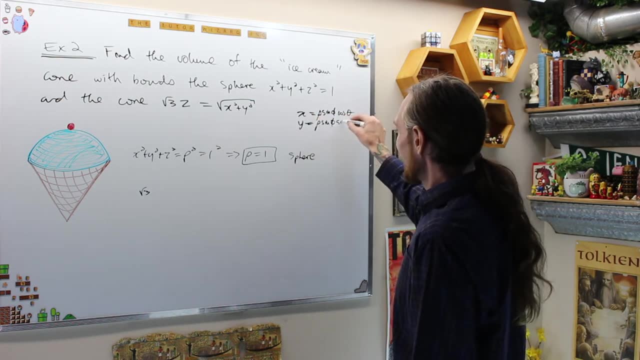 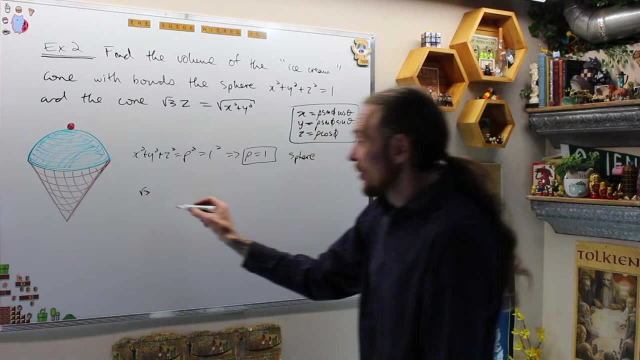 to be root 3. and what is z, remember? x is rho sine phi cos theta, y is rho sine phi sine theta and z is rho cos phi. so I'm putting those in here now. this is root 3: rho cos phi equals the square root rho. 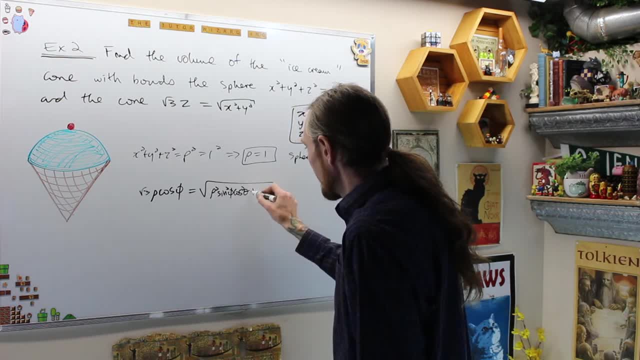 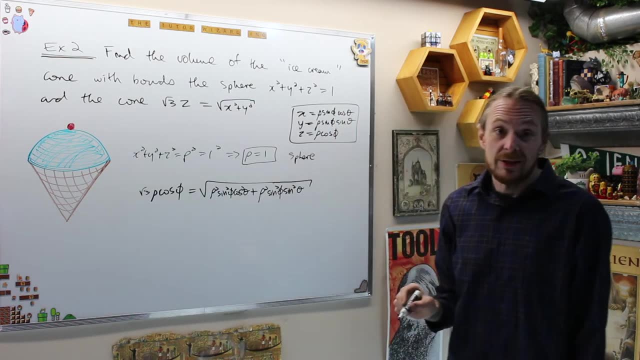 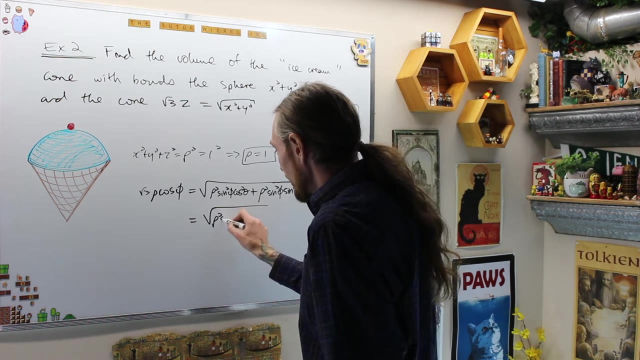 squared sine squared phi cos squared theta, plus rho squared sine squared phi sine squared theta. oh, I can just smell a trigonometric identity. I have rho squared sine squared phi in both terms. I'm going to factor that out. that's going to give me the square root of rho squared sine squared b times cos squared. 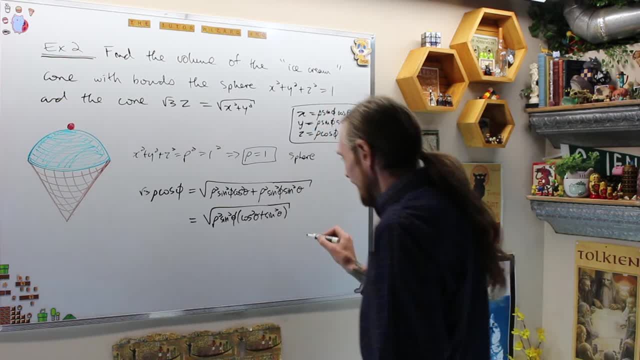 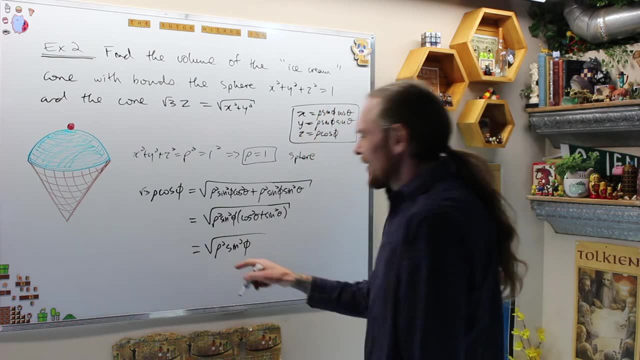 theta plus sine squared theta. pavlov is already biting at the biscuit. this is going to be the square root, this is one. this is the square root of rho squared sine squared phi. technically rho, because he's a radius, and sine phi in here is going to be positive in our quadrant that we're in. 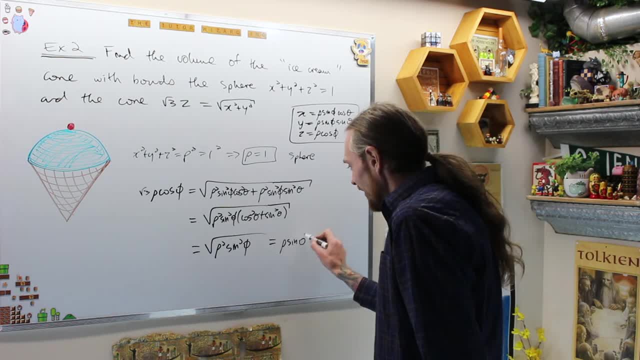 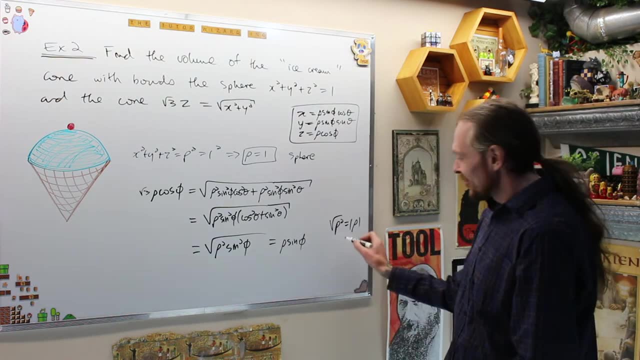 we've checked. so this is going to give me a rho sine phi. still, I still did a little thing. I'm gonna square root squared and the square root of ro squared is absolute value rho. but I was like he's positive, so don't worry, I could get rid of it. that's what I was doing every time, every. 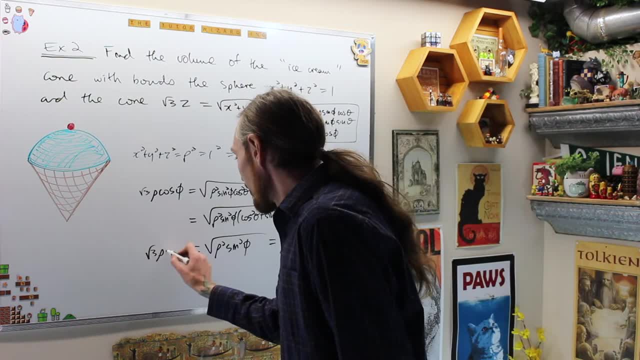 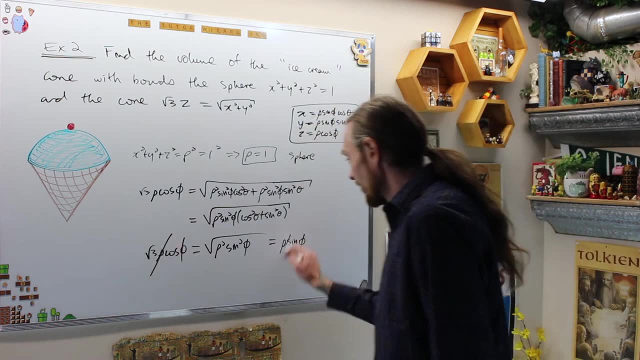 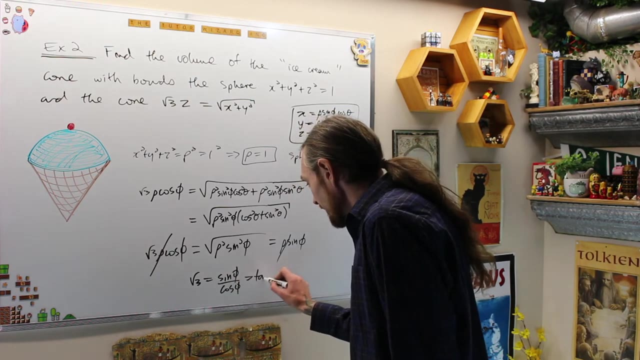 time. now that simplifies. that tells me that root 3, rho cos phi equals rho sine phi. I can cancel row first of all, and he's non-zero, and then I get what root 3 is equal to sine B over cos B, which is tan of B, and that is going to tell me that my equation is: 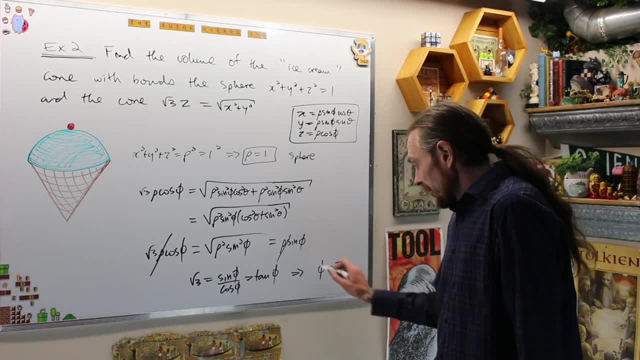 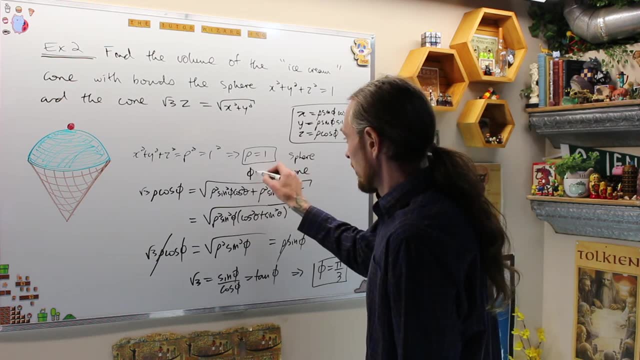 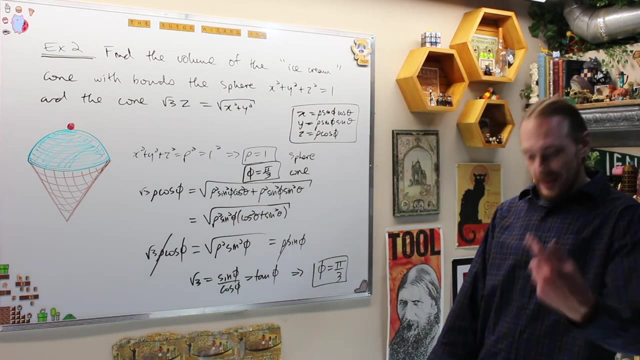 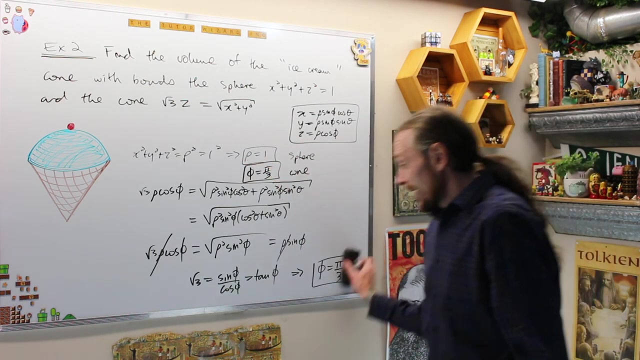 going to be what? B is equal to pi over 3. that's the equation of the cone, much nicer. and there's the practice of how to switch back and forth between rectilinear or Cartesian and spherical. now we're going to use that information to describe our bounds and everything. what do we have now, therefore? our bounds. 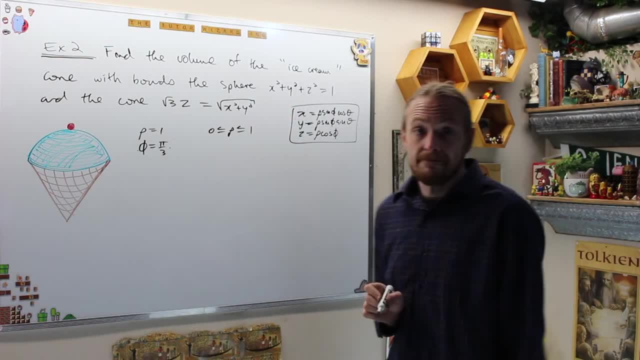 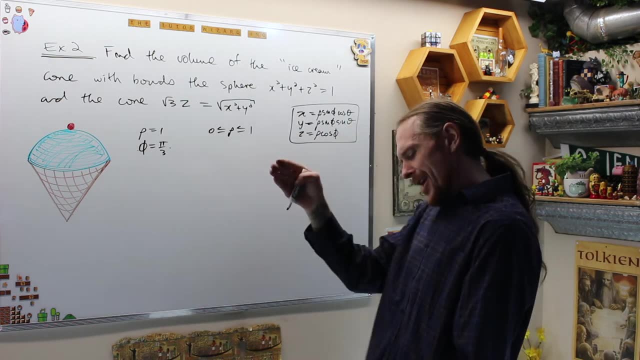 this says 0 is less than or equal to rho is less than or equal to 1. this says that we're going all the way around because I want to eat the whole ice cream cone. I'm not cutting it out of you. shit you can't share with Timmy. I don't want to, so you. 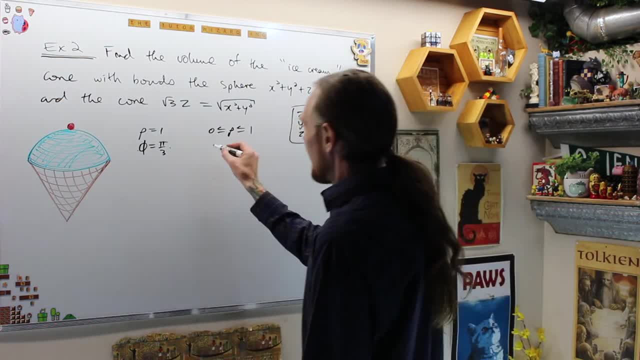 get, everyone has to get a whole one. I guess I'll figure out how to do that. and then what are we going to get? 0 is less than or equal to theta, less than or equal to 2 pi all the way around. and then 0 is less than or equal to. 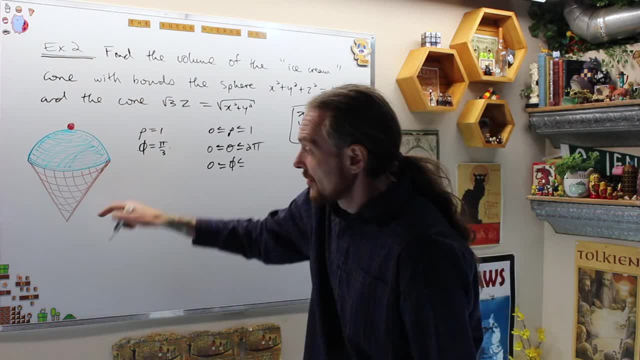 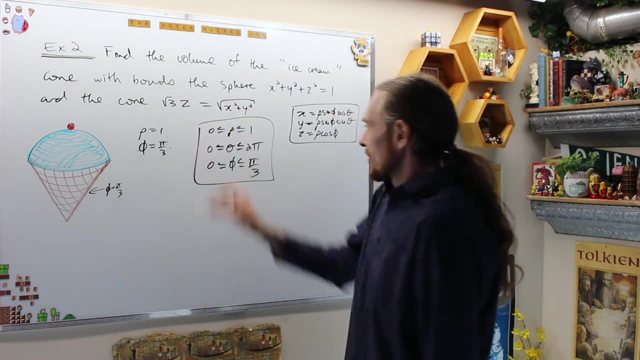 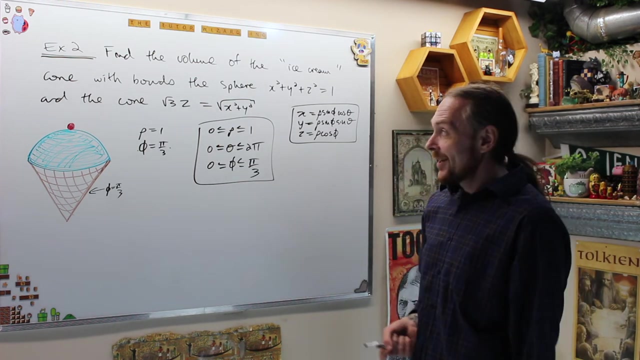 to b and we're going to stop at our bounds right here, which is this guy is b equals pi over three, so we have pi over three. all those looks so it's like numbers, numbers, numbers. try and do that in rectilinear, not numbers. i'll tell you that right now and then what is that going to give us? that's. 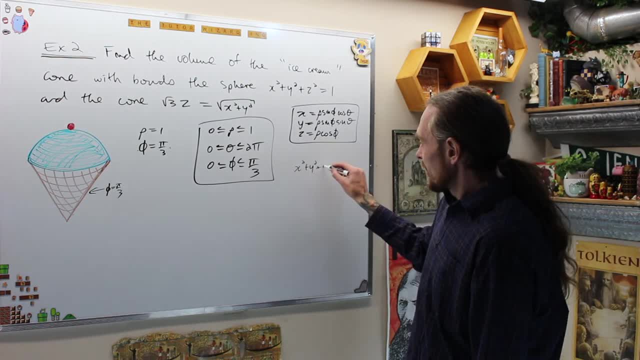 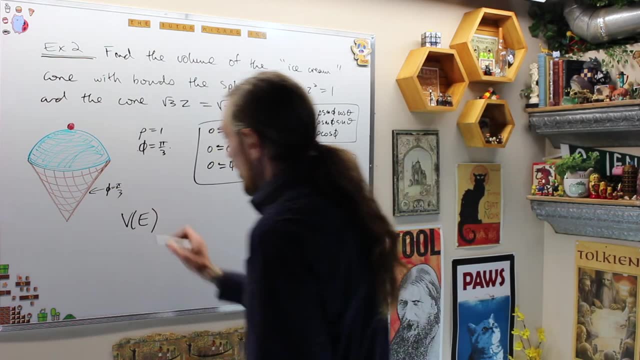 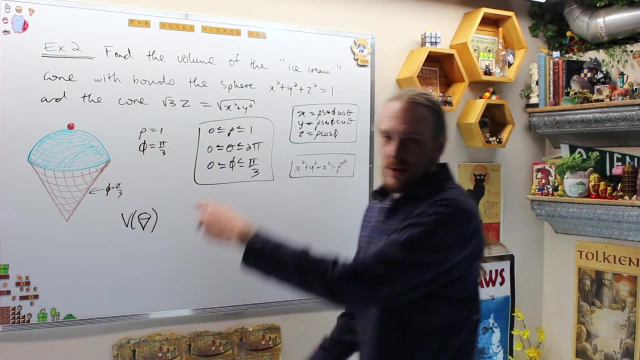 now going to give us and remember, x squared plus y squared plus z squared equals rho squared also all the time. therefore, the volume of this object e, which is our ice cream cone, even we can put single painted algebra, the cherry is not involved in there. the cherry's volume is fourth roots pi. 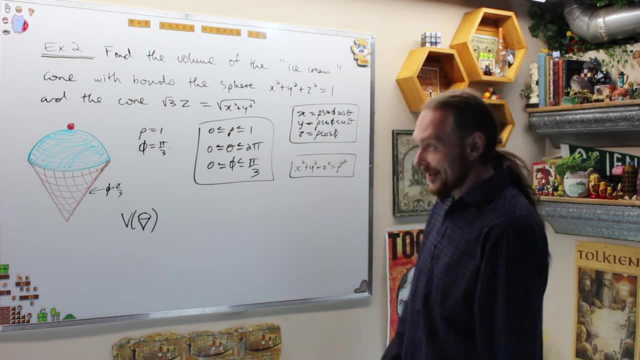 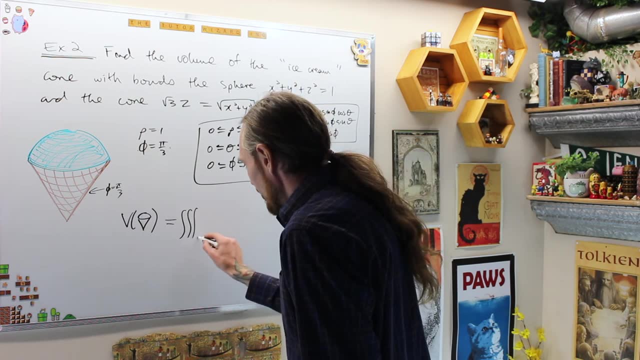 r cubed, where the r is the radius of the cherry. you can do that one at a different video. eat the cherry first, then we're going to eat the ice cream gang. the volume of this is equal to the triple integral over e, dv, which is best phrased in spherical coordinates. that's going to be the. 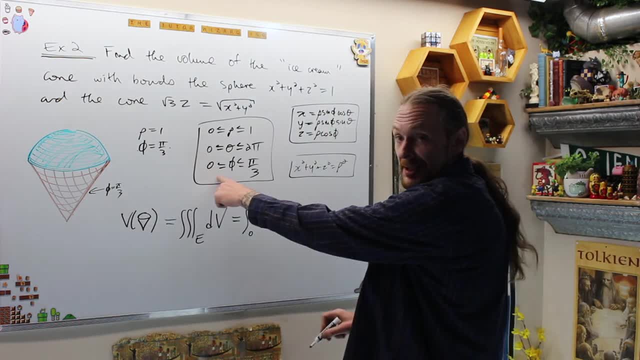 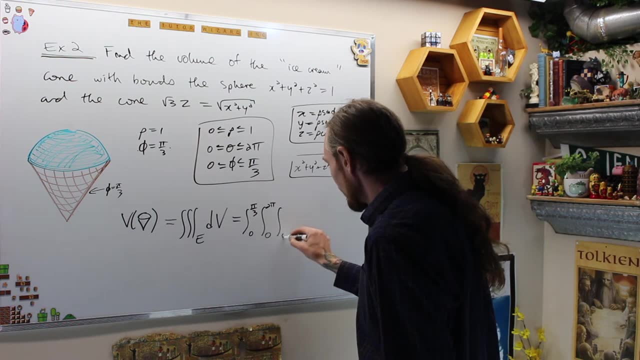 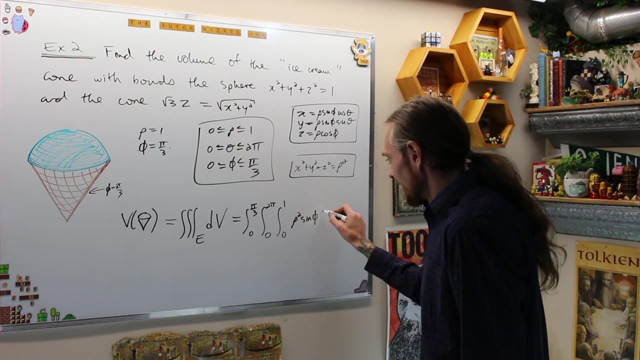 integral from you, the integral from zero to pi, over three him first, because it's d? rho d theta d, phi is how i set this up. and then so the integral from zero to two, pi the integral from zero to one. uh, now, what do we get? don't forget the rho squared sine b, d rho d theta d c. that guy's always going to be there. so 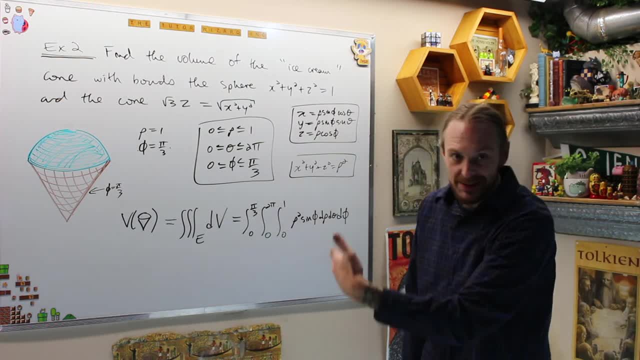 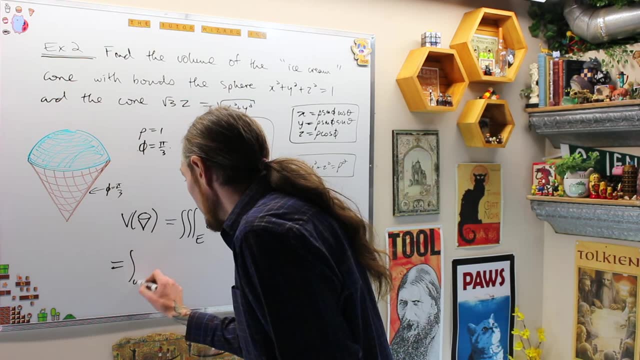 now, you're always going to be integrating. hopefully you get one over a sine b, because then it'll cancel, but you're always going to be integrating the fees. finally, for once in a while, this is going to give me equals: the integral from zero to pi over three, the integral from zero to two. 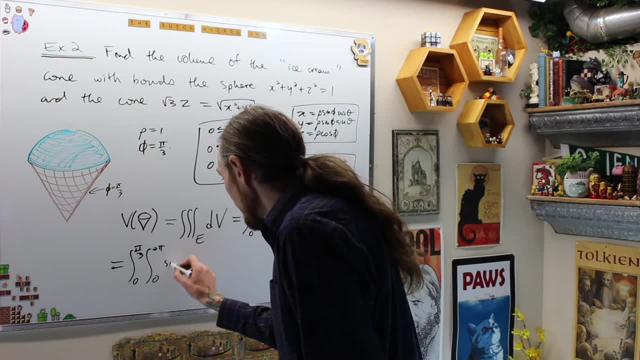 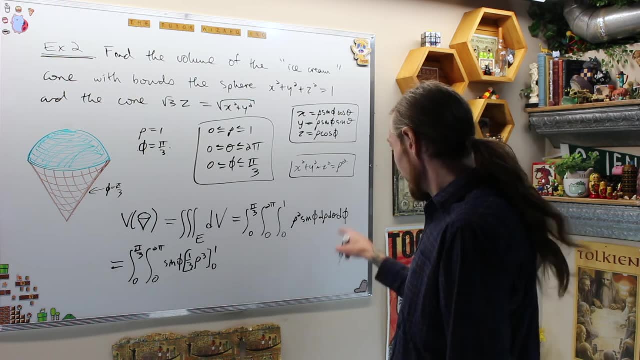 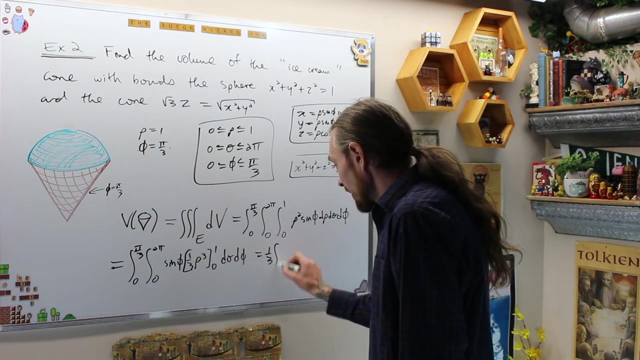 pi. i'm doing d rho first, so that is going to give me sine one third. rho cubed evaluated from zero to one. oh, i like that you should see the bounds in cartesian d theta d phi. this is going to give me one third. this gives me one third. the integral from zero to pi over three. the integral from zero. 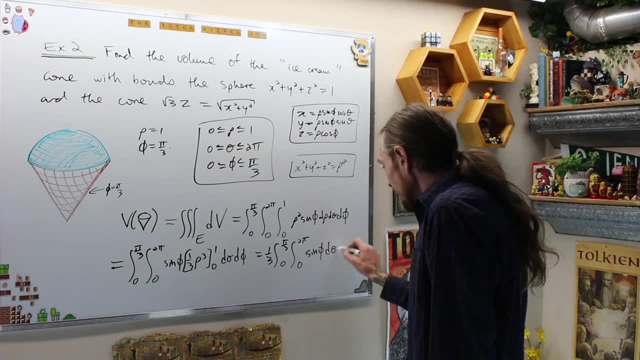 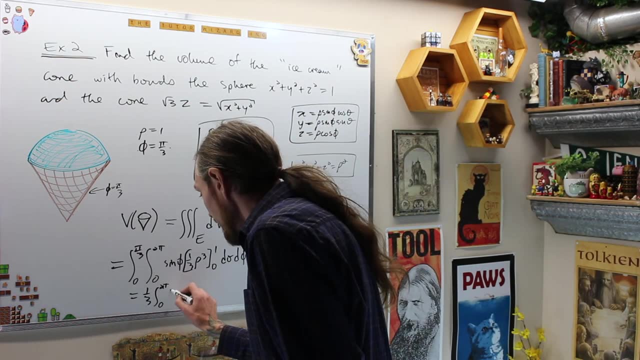 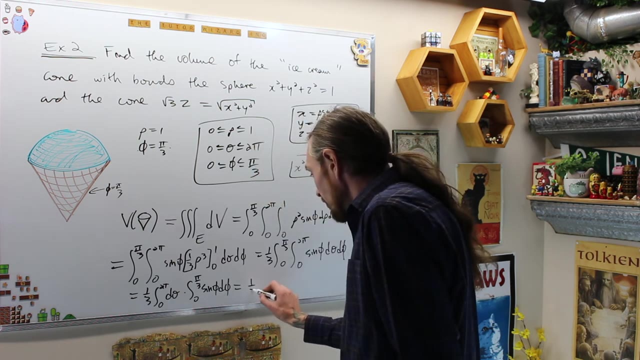 to two pi of sine b d theta d phi. these are now separated so i'm going to. this is equal to one third the integral from zero to two pi of d theta times the integral from zero to pi over three of sine b d phi, which is equal to one third times two pi times. this one is negative. cos phi evaluated.